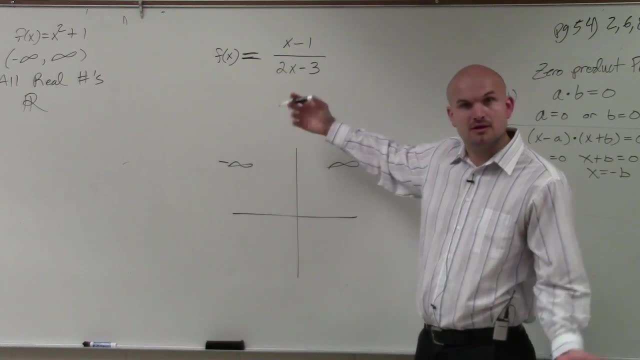 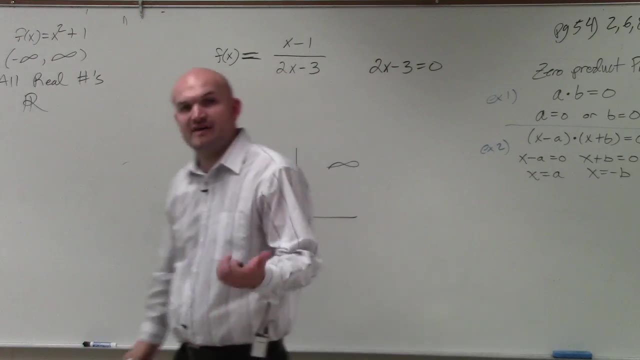 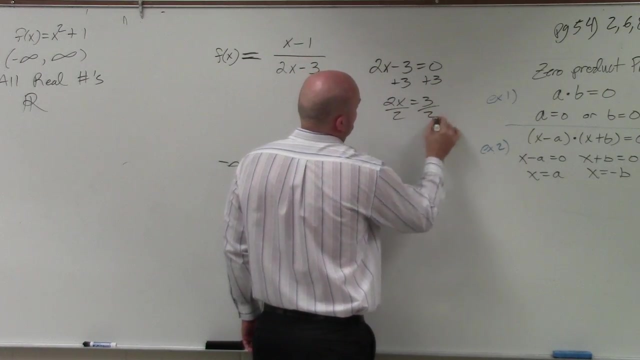 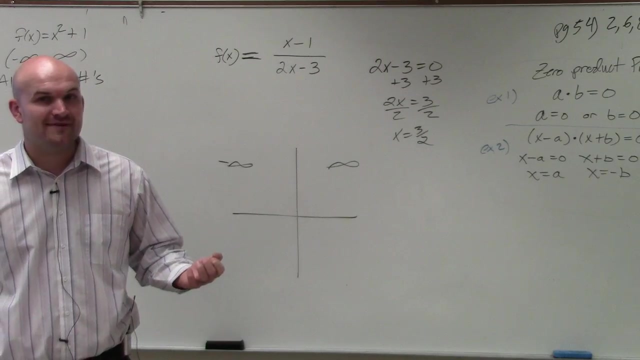 what number then makes my denominator equal to zero? Well, the easiest way to do that is to take out the denominator and just set it equal to zero, so I can find the value of X. that does that So using our inverse operations from algebra. X equals three halves. So that means when X is equal to three halves, when X is equal to three halves, that makes my denominator zero. So 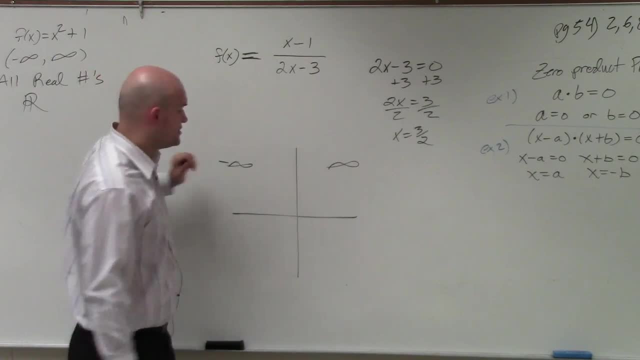 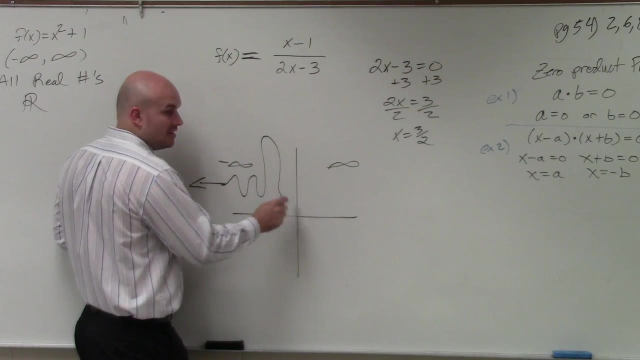 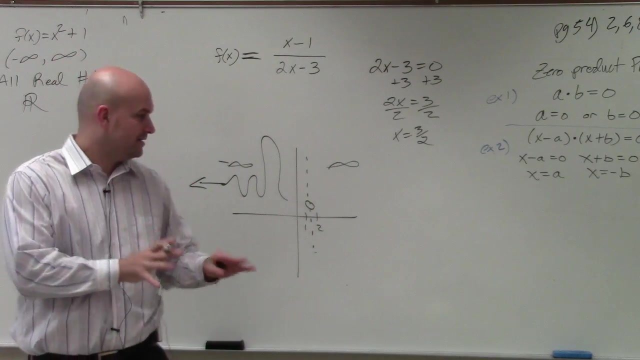 guess what? Three halves is not inside the domain. So we have our function. Our function goes all the way to infinity. It can do whatever stuff it wants to do. But at three halves, here's one, here's two. three halves is like right here, At three halves there's either a whole or an asymptote. We don't know what it is right now. We're going to learn about how to determine your asymptotes and holes later, But for right now you can just say this function: continue is continuous. 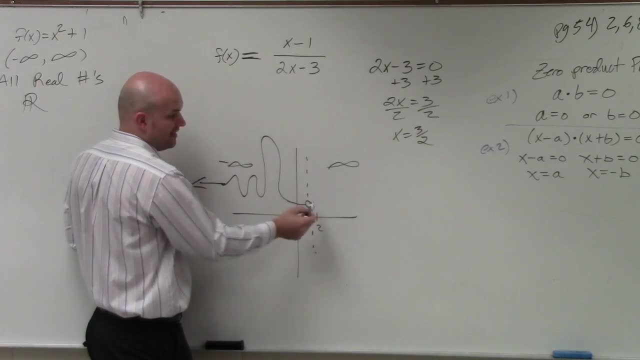 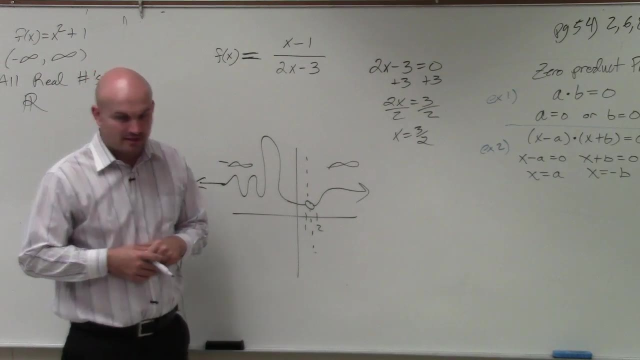 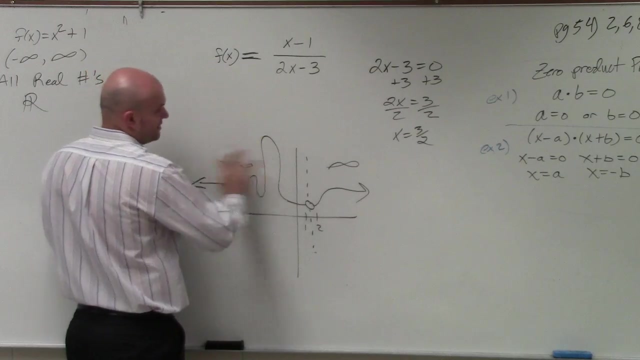 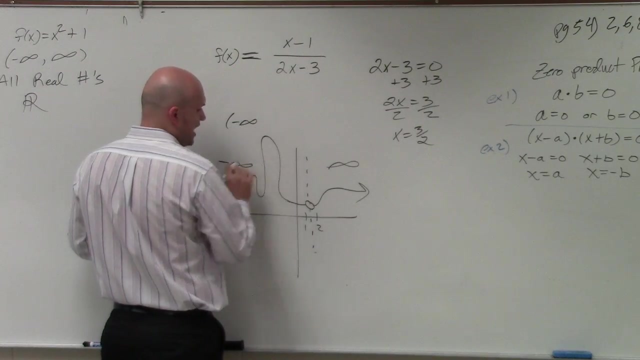 Except it doesn't include the value three halves. And then it continues from there. So it's all real numbers except for that value. Now I want to show you guys how to write that in interval form, because we wrote all real numbers as negative infinity to infinity, But in reality this is going from negative infinity to how far over does it go? 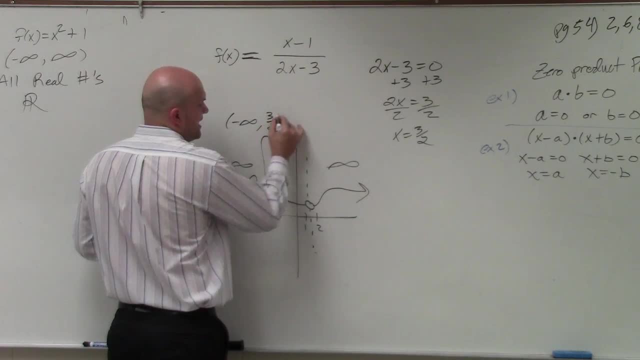 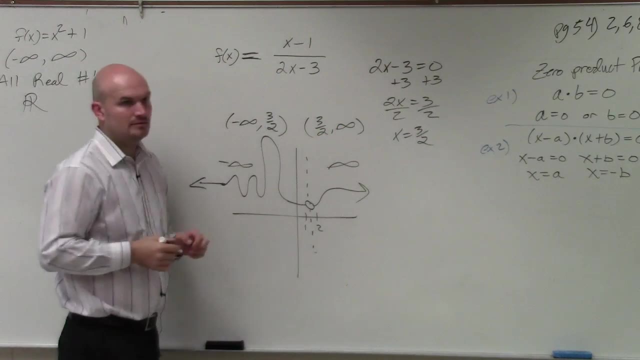 until it has to stop To three halves. Then it starts back. that starts back up again from 3 1⁄2 to infinity, Do you guys kind of agree? And it doesn't include 3 1⁄2, so that's why it's a parentheses. 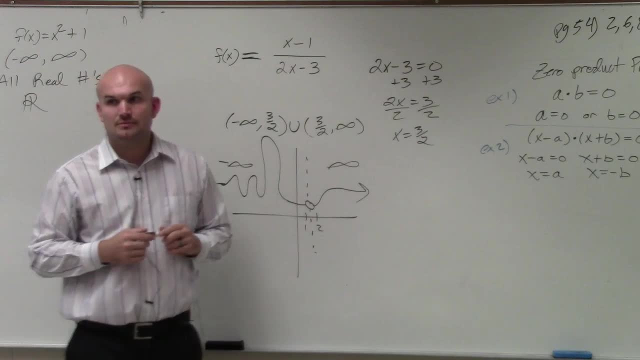 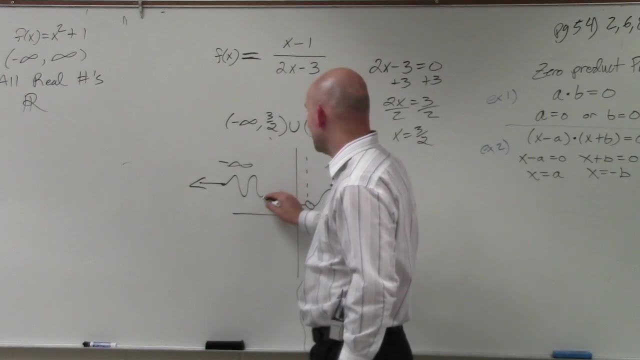 So to connect these we use the union symbol. Yes, It's just me telling you it's like a made-up graph. I mean, I don't know what the graph looks like. It's definitely a function, but we don't know what the graph looks like. 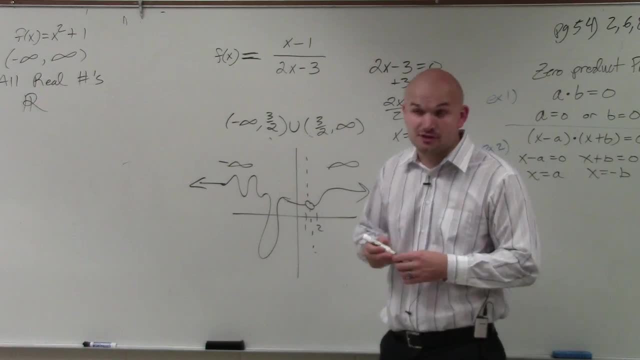 It's probably something easy, right? It's not going to be something crazy, And actually let's go and take a look at the graph to make sure that makes sense. So we will be practicing this next class period.